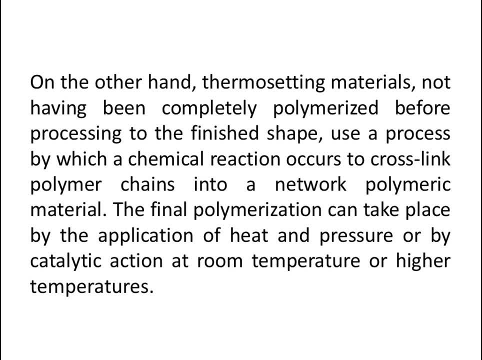 On the other hand, thermosetting materials not having been completely polymerized before processing to the finished shape use a process by which they are used. On the other hand, thermosetting materials not having been completely polymerized before processing to the finished shape use a process by which they are used. 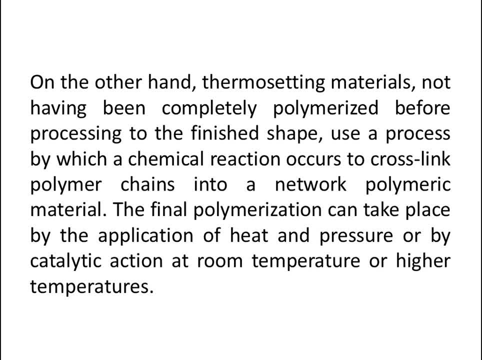 On the other hand, thermosetting materials, not having been completely polymerized, before processing to the finished shape, use a process by which they are used. A chemical reaction occurs to cross-link polymer chains into a networked polymeric material. The final polymerization can take place by the application of heat and pressure, or by catalytic action at room temperature or higher temperatures. 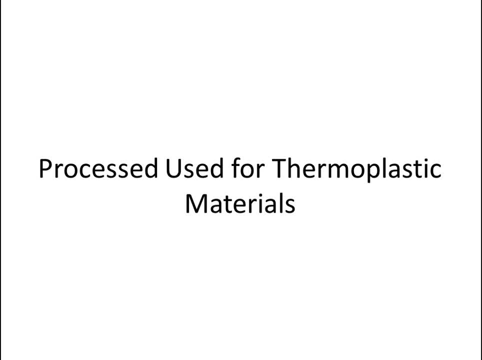 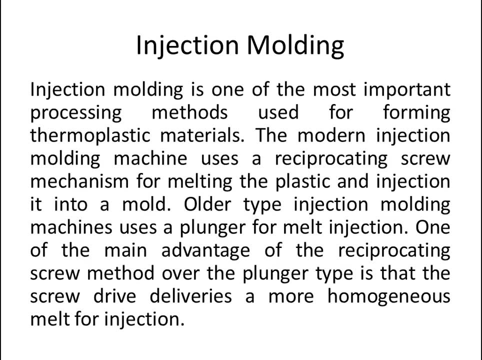 Now let's talk about the process used for thermoplastic materials, And first one is the injection molding. Now let's talk about the process used for thermoplastic materials. Actually, injection molding is one of the most important processing methods used for forming thermoplastic materials. 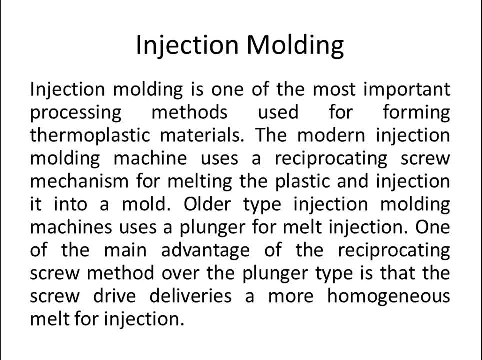 The modern injection molding machine uses a reciprocating screw mechanism for melting the plastic and injection it into a mold. Older type injection molding machines uses a plunger for melt injection. One of the main advantages of the injection molding is that it can be used for melting plastic into a mold. 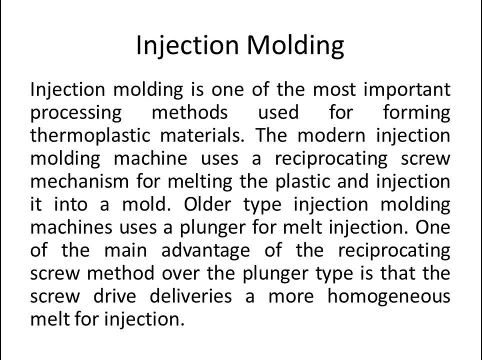 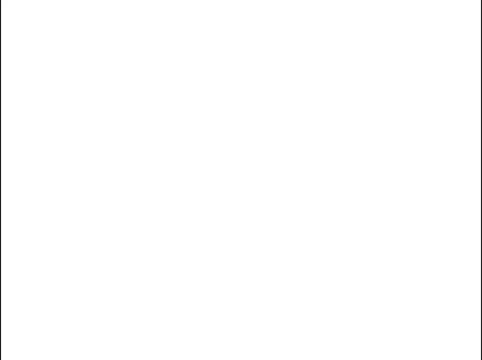 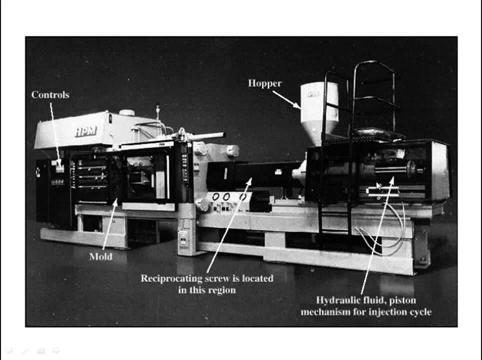 reciprocating screw method over the plunger type is that the screw drive deliveries are more homogeneous: melt for injection and there is a picture for this one, and at this side there is hydraulic fluid and piston and there is hopper. so through this hopper the material is a permitted to allow to go. 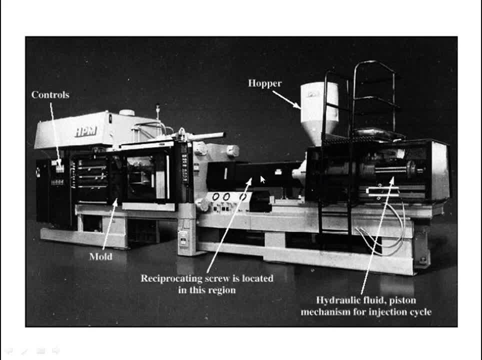 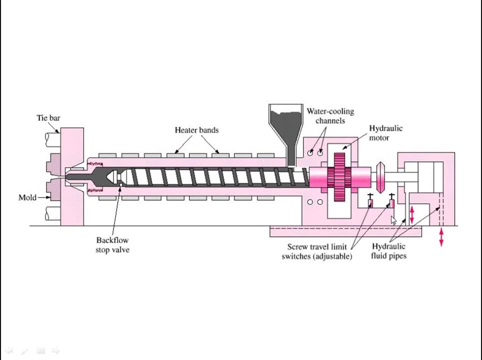 to the machine and here is the reciprocating screw. and here is the mold, is actually liquid up situated here and the machine is controlled from here and there is a cross-section view. so there is the hydraulic fluid pipe and there is screw, and there is this one is the hydraulic hydraulic motor and water. 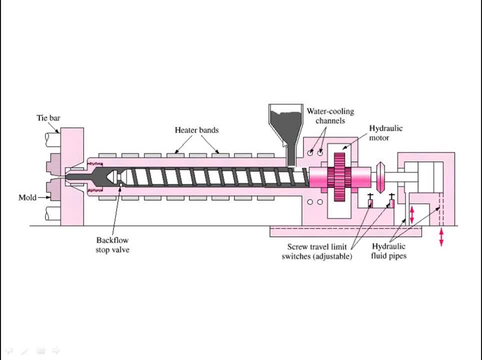 cooling channels are actually here. so there is a hopper, and this hopper contains the material, and this hopper contains the material, and this hopper contains the material. and these are the heater bands. and here these are the heater bands. and here these are the heater bands. and here there is black flow stop valve and the 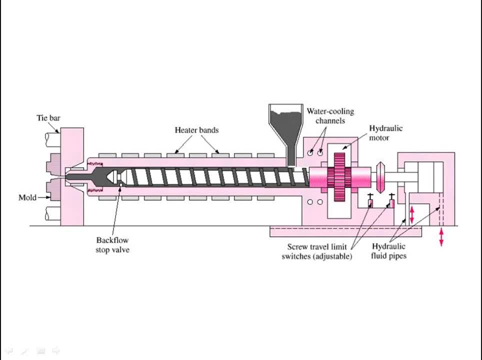 there is black flow stop valve and the there is black flow stop valve and the mold is actually there. the molds and mold is actually there. the molds and mold is actually there. the molds and there is Tiber and there is a step by. there is Tiber and there is a step by. 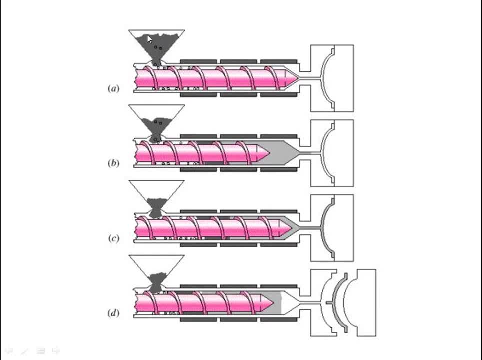 there is Tiber and there is a step by step figure. so initially there is the step figure, so initially there is the step figure. so initially there is the material and the mold is here. so material and the mold is here. so material and the mold is here. so materials are coming and the materials 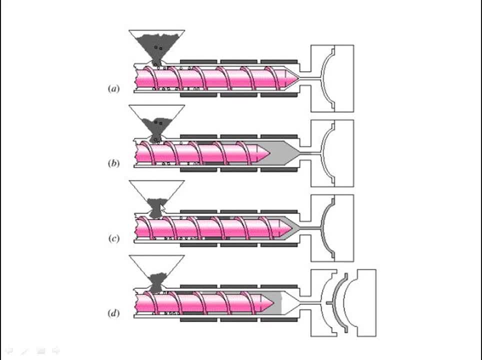 materials are coming and the materials. materials are coming and the materials are going, traveling this way. and as the are going traveling this way, and as the are going traveling this way, and as the materials are decreasing, materials are decreasing, materials are decreasing and the materials are going. and now the mold. 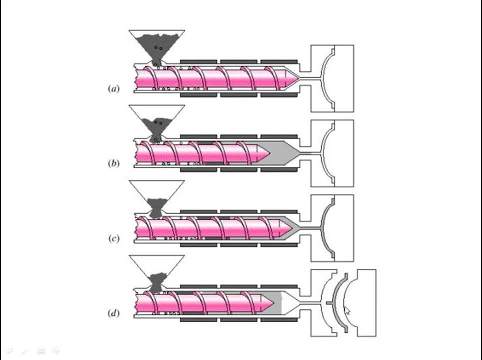 and the materials are going, and now the mold and the materials are going, and now the mold is filled by the material and finally is filled by the material and finally is filled by the material. and finally, when the mold is filled, the one, what is? when the mold is filled, the one, what is? 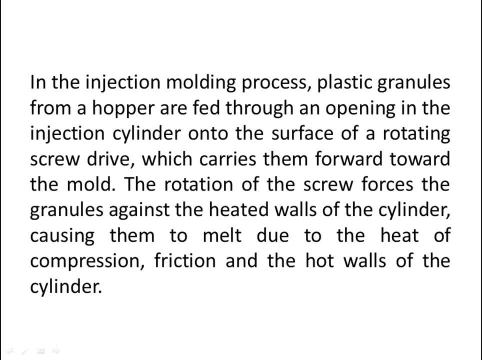 when the mold is filled, the one, what is isolated from here, literally in the isolated from here, literally in the isolated from here, literally in the injection molding process. plastic injection molding process. plastic injection molding process. plastic granules from a hopper are fed through an. granules from a hopper are fed through an. 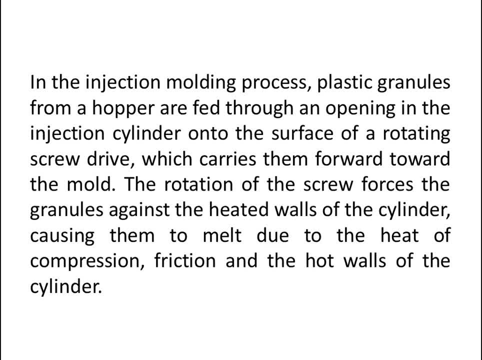 granules from a hopper are fed through an opening in the injection cylinder onto opening in the injection cylinder, onto opening in the injection cylinder onto the surface of a rotating screwdriver. the surface of a rotating screwdriver which carries them forward toward the mold. the rotation of the screw forces. 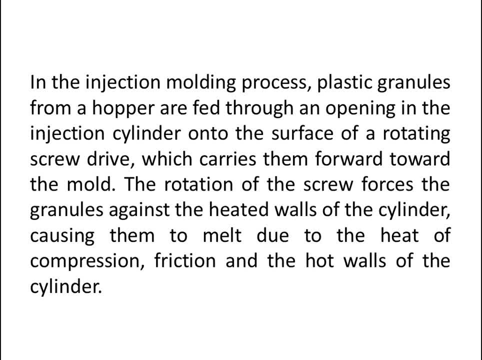 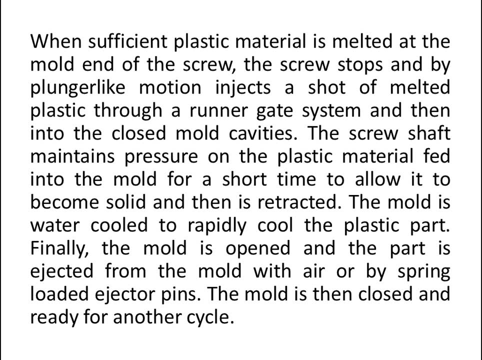 the granules against the heated walls of the cylinder, causing them to melt due to the heat of compression, friction and hot walls of the cylinder. when sufficient plastic material is melted at the mold end of the screw, the screw stops and by a plunger like motion injects a shot of melted plastic through a runner gate. 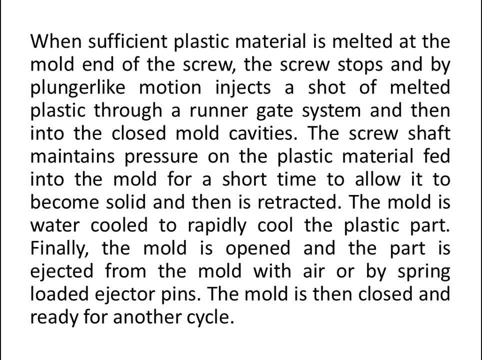 system and then into the closed mold cavities. the screw shaft maintains pressure on the plastic material, fade into the mold for a short time to allow it to become solid, and then is retracted. the mold is water cooled to rapidly cool the plastic part. finally, the mold is open and the part is ejected from the 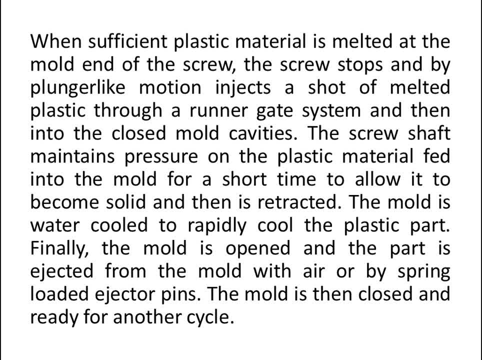 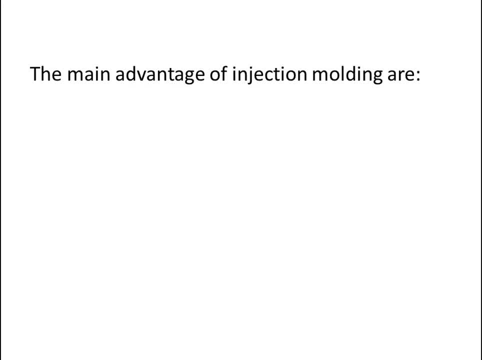 mold with air or by spring-loaded ejector pins. the mold is then closed and ready for another cycle. the main advantage of injection molding are: first one: high quality parts can be produced at a high production rate. second one: the process has relatively low labor cost. third one: good surface finishes can be. 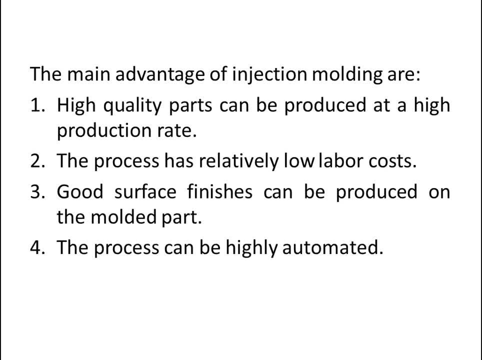 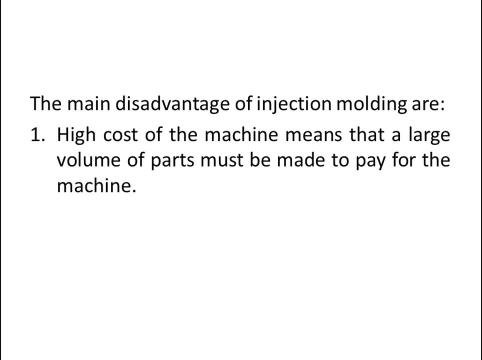 produced on the molded part. fourth one: the process can be highly automated. and fifth one: intricate shapes can be produced. the main disadvantage of injection molding are: first one: high cost of the machine means that a large volume of parts must be made to pay for the machine. second one: the process must. 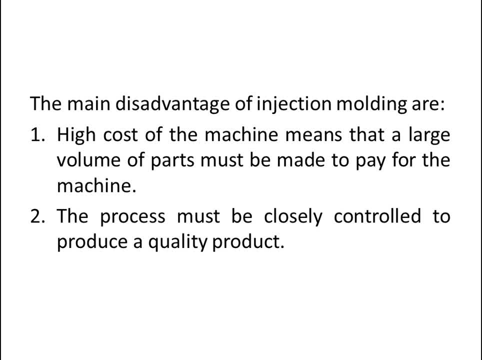 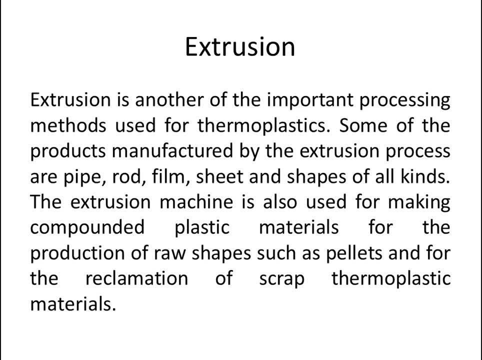 be closely controlled to produce a quality product. now let's talk about the extrusion process. extrusion is another of the important processing methods used for thermoplastics. some of the products manufactured by the extrusion process are pipe, rot film sheet and shapes of all kinds. the extrusion machine is also. 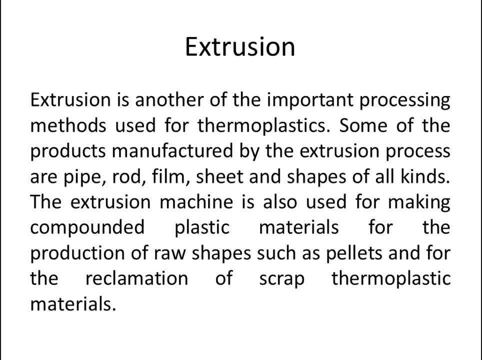 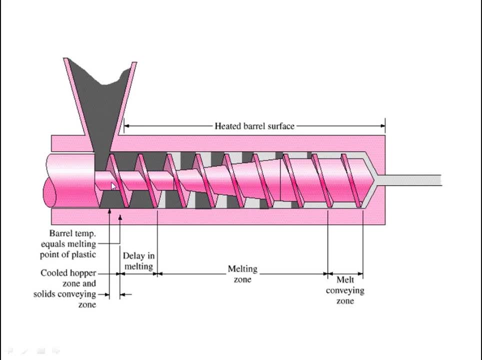 used for making compounded plastic materials, for the production of raw shapes such as pellets and for the reclamation of scrap thermoplastic materials. and as a picture for this one. so there is the hopper and through this hopper the material actually come and they travel in this way. so the first, 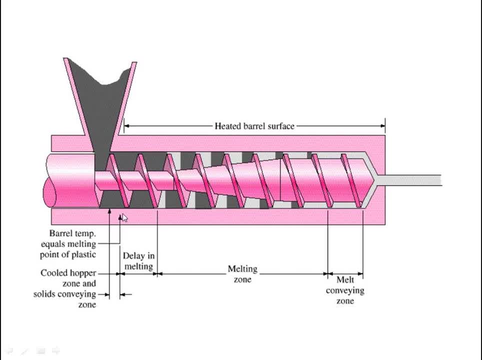 portion is the cooled hopper zone and solid conveyor zone and this portion is the barrel. temperature equals melting point of plastics and between this portion is the delivery in melting and this portion is the melting zone. and finally, this portion is melt conveying zone and the upper portion is the heated. 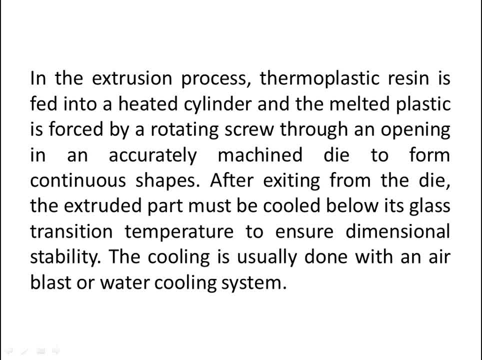 barrel surface. now, literally in the extrusion process. thermoplastic resin is fed into a heated cylinder and the melted plastic is tossed by a rotating screw through an opening in and accurately mesh in die to form continuity shapes. after exciting from the die, the extruded part must be cooled below its 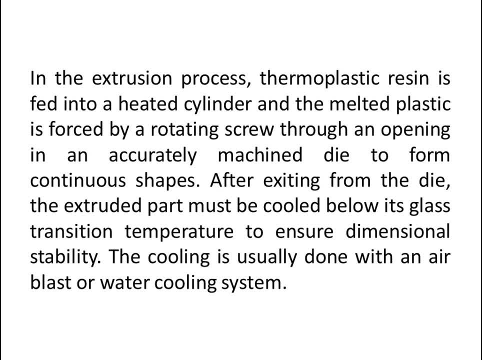 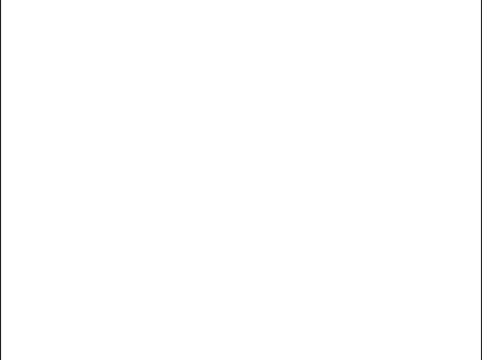 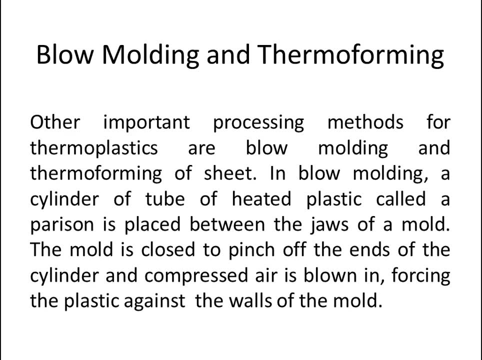 glass transition temperature to ensure dimensional stability. the cooling is usually done with an air blast or water cooling system. now let's talk about blow molding and thermo forming, other important processing methods for thermoplastic or blow molding and thermo forming of sheet. in blow molding, a cylinder of cube of heated plastic called a parison is placed between the 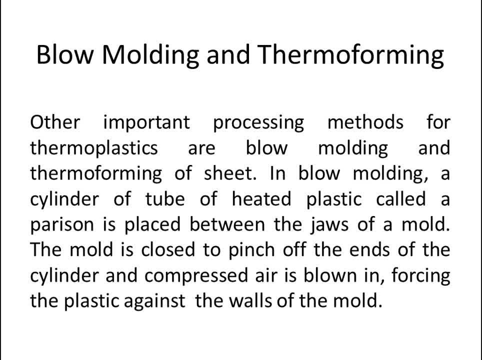 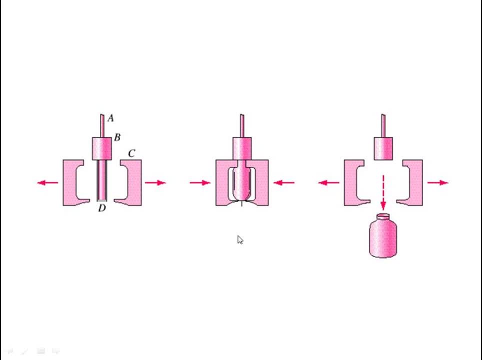 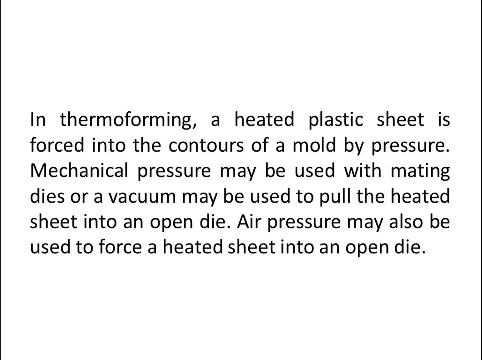 jaws of a mold. the mold is close to pinch of the ends of the cylinder and compressed air is blown in, forcing the plastic against the walls of the mold and there's a picture for this one. so there are three pictures identifying them. literally, in thermal forming, a heated plastic sheet is forced into the. 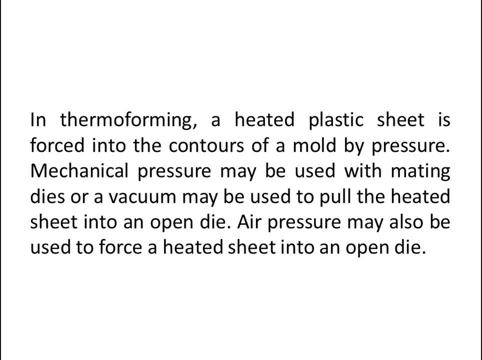 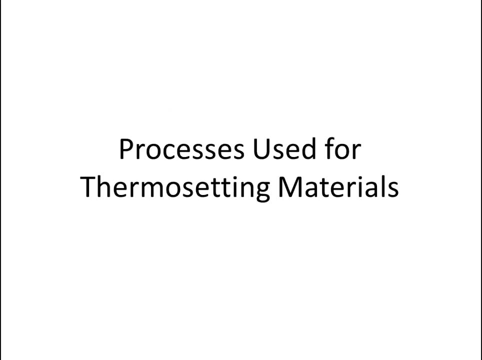 counters of a mold by pressure. mechanical pressure may be used with metting dies or a vacuum may be used to pull the heated sheet into an open day. your pressure may also be used to force a heated sheet into an open day. now let's talk about used for thermosetting materials, and first one is the compression molding. 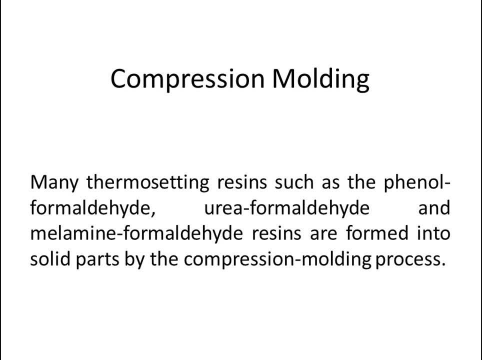 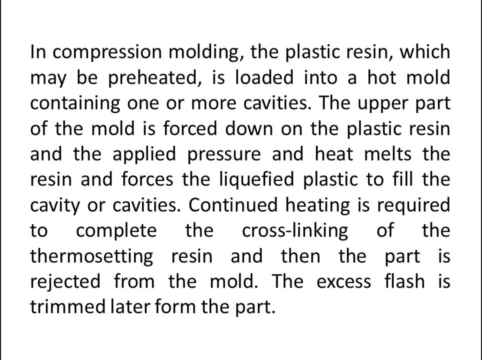 process. many thermosetting resins, such as the phenol, formaldehyde, urea, formaldehyde and melamine formaldehyde resins are formed into solid parts by the compression molding process. in compression molding, the plastic resin which may be preheated is loaded into a hot mold containing one or more cavities. 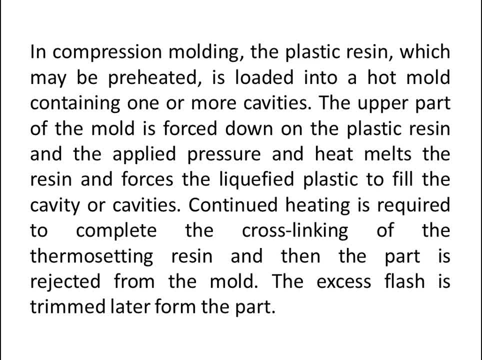 the upper part of the mold is forced down on the plastic resin and the applied pressure and the and heat melts the resin and forces the liquefied plastic to fill the cavity or cavities. continuous heating is required to complete the cross linking of the thermosetting resin and then the part is. 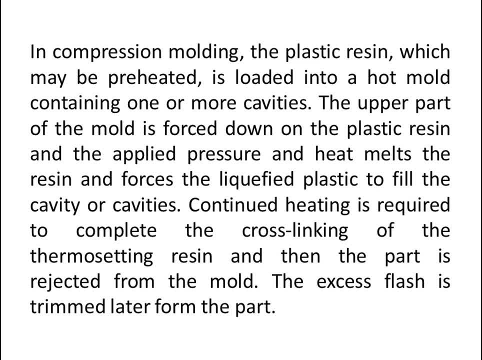 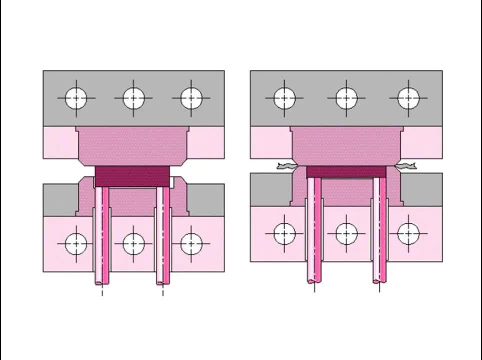 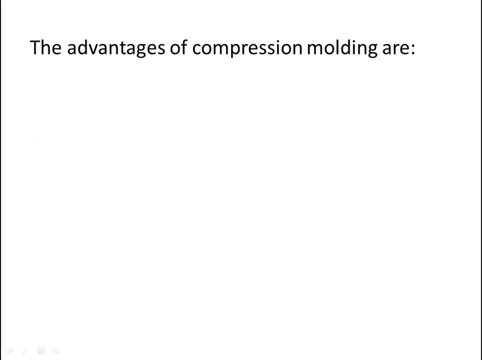 rejected from the mold. the excess flash is trimmed later from the part. and there are two figures. the first one is the open molding system and second was the closed molding system. the advantages of compression molding are: first one: because of the relatively simplicity of the molds, initial mold cost are low. second one, the relatively 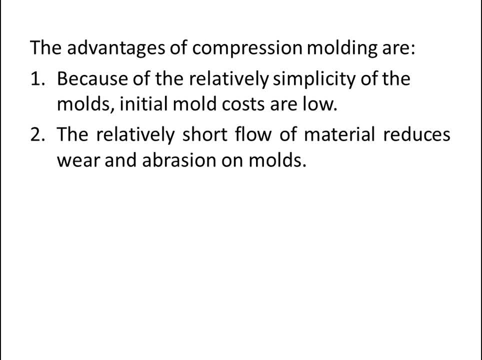 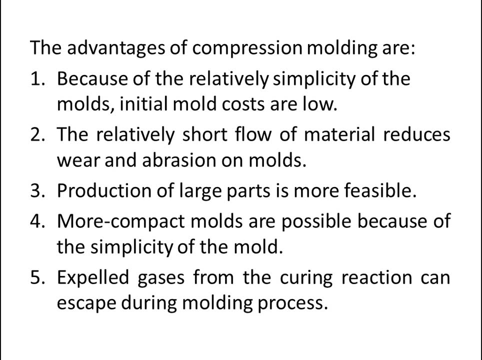 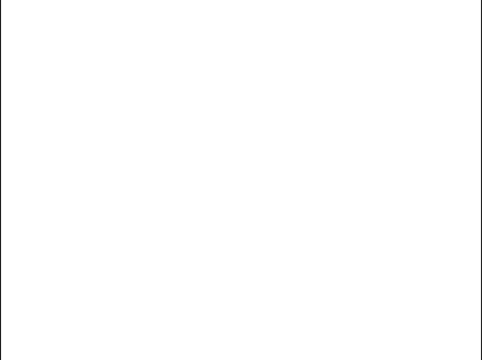 short flow of material reduces wire and abrasion on molds. third one: production of large parts is more feasible. fourth one: more compact molds are possible because of the simplicity of the mold. fifth one: expelled gases from the curing reaction can escape during molding process. on the other hand, the 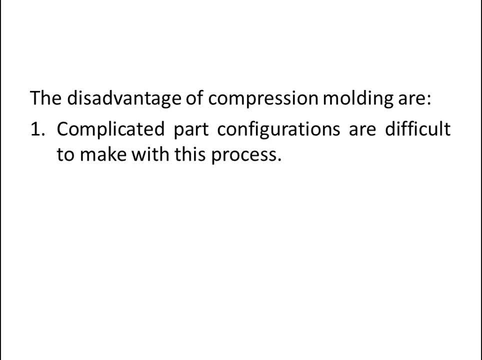 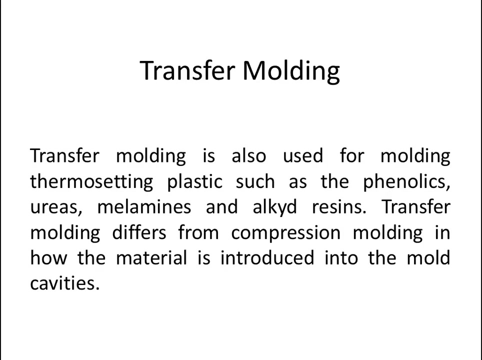 disadvantages of compression molding are already explained by our use of labor force for WILL. first, one complicated part configurations are difficult to make with this process. second, one incest may be difficult to hold two closed tolerances. third, one flash must be trimmed from the molded parts. now let's talk about transfer molding. transfer molding is also used for molding thermosetting plastics such as the phenolix, euryas, melamine and alloy ma deficiencies. 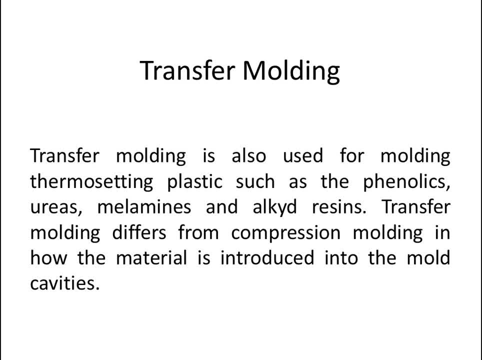 transfer molding is also used for molding thermosetting plastics such as the phenolix, eury, Sellam, us and, after the molding process, ERE are of multiple strength are out there in the avec Обity technology and alkyd resins. transfer molding differs from compression molding in how? 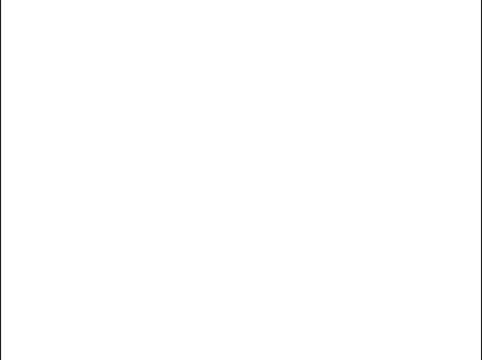 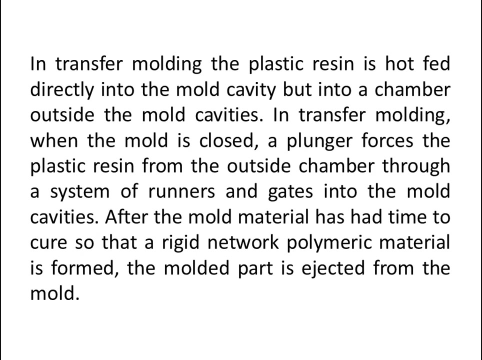 the material is introduced into the mold cavities. in transfer molding the plastic resin is hot fit directly into the mold cavity but into a chamber outside the mold cavities in transfer molding. when the mold is closed, a plunger forces the plastic resin from the outside chamber through a system of runners and gets. 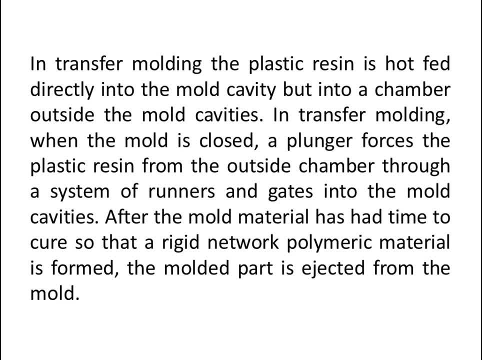 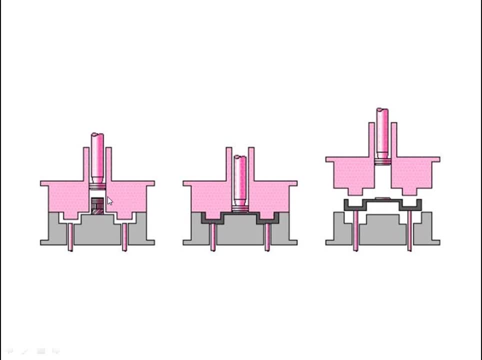 into the mold cavities. after the mold material has had time to cure, so that a rigid network polymeric material is formed, the molded part is ejected from the mold. and there's a picture for this one, three pictures actually there. so first one. so here is the material. so when it is compressed it is distributed.